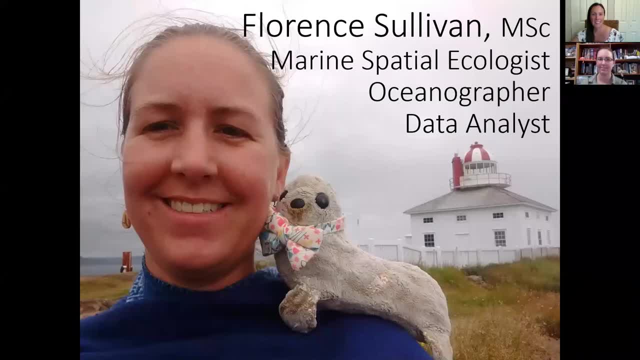 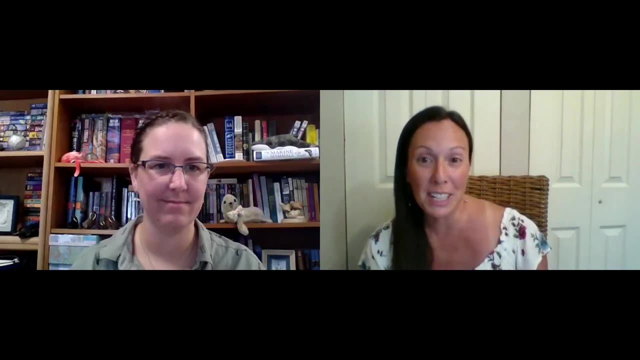 All right, Good morning everyone. Thanks so much for joining us for another episode of our Careers in Marine Science and Ocean Conservation series. My name is Robin Ehrlich. I'm the Education Manager at Pacific Whale Foundation. Today I've got Florence Sullivan here with me, our Research Analyst. 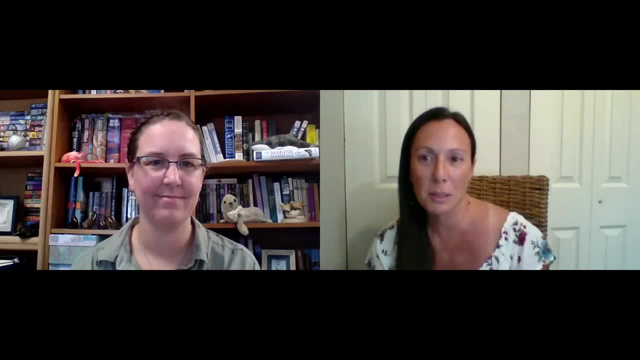 And this series, I'm hoping, is a fun way for everybody to get to know some of our team members in a different way. So we often get to meet team members and find out about what they currently do, But not so much the pathway that got them to where they are. 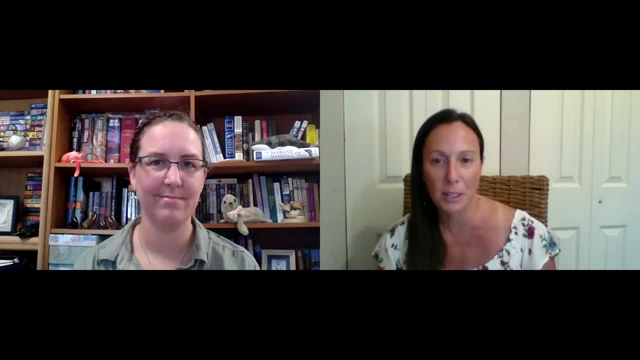 And I know a lot of people that come in contact with Pacific Whale Foundation or PacWhale EcoAdventures are often inspired to work with us and wonder what it takes to get to a position like this, And a lot of our team members have these really interesting career journeys that got them to where they are. 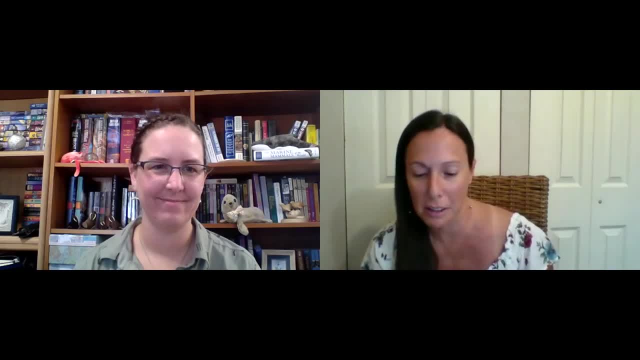 And so I hope this is interesting and inspiring for everybody to learn about. And we've all kind of started from some pretty unique career goals as children, And Florence certainly has a unique story. So I want to introduce Florence Sullivan and let her tell us a little bit about herself. 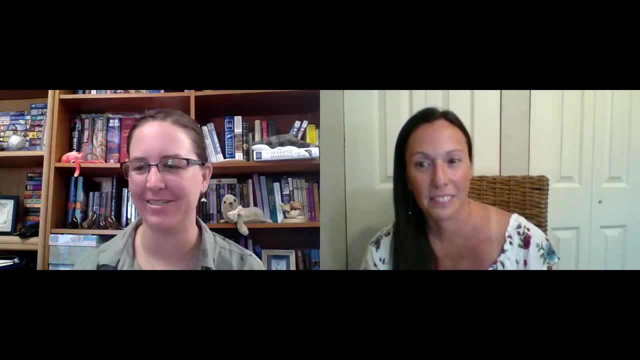 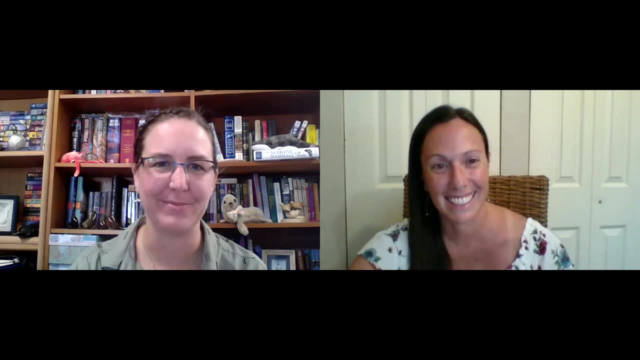 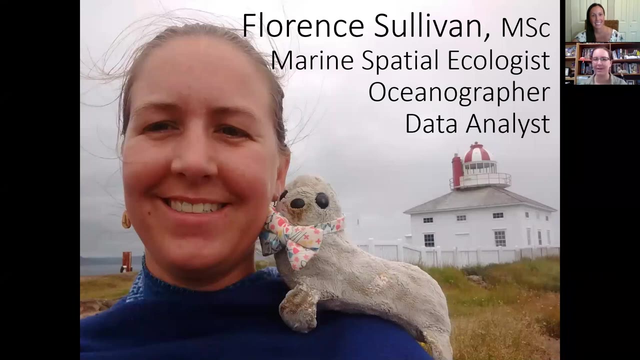 All right, Hi everyone. Thanks so much for joining us today. I have made a little PowerPoint with lots of photos that hopefully won't be too embarrassing, to help share my story. Thanks, Robin, for the lovely introduction. As she said, my name is Florence Sullivan. 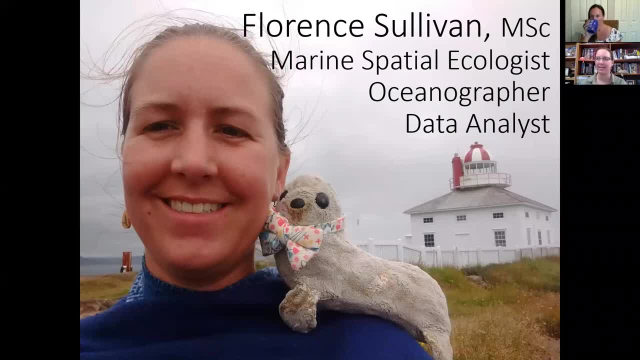 I have had. Sorry. let me gather my thoughts here. What's really cool about this series of webinars that Robin's put together is, once you start talking to those of us in the field, you realize no one has had a straight path. 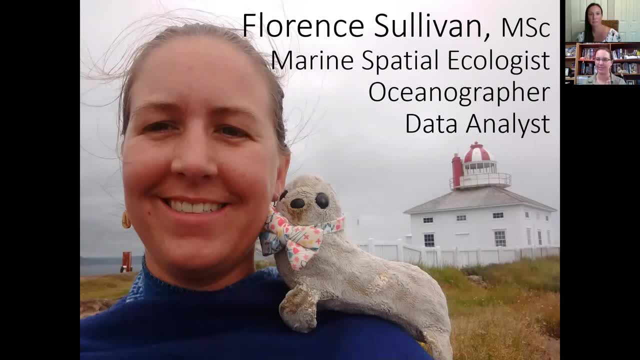 No one knows exactly how they're going to get to where they're going. Or, And As you can see on this slide here, I've got a couple of different career fields that I sort of consider myself part of. I started as an oceanographer. 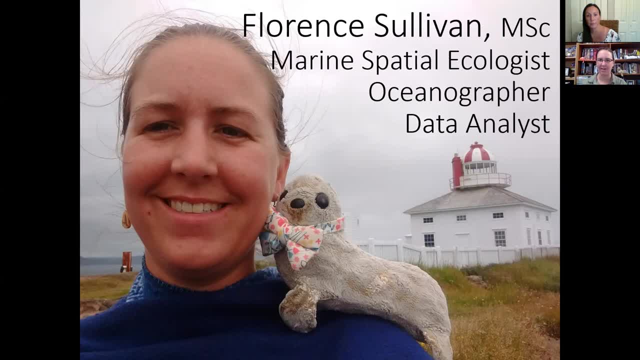 I have spent time as a marine spatial ecologist, And let's break those big words down for a second. Marine means everything related to the ocean, right? Spatial is how things move through space And ecology is The big puzzle of how the world goes together, right? 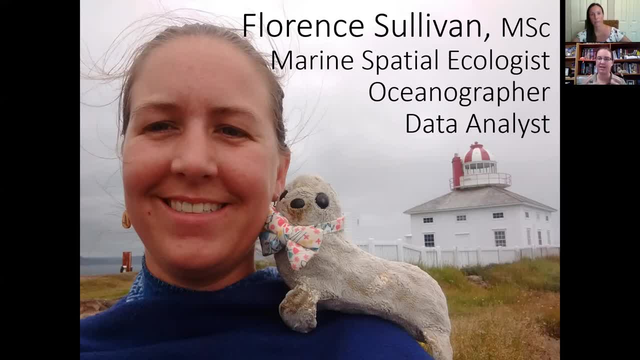 So, as a marine spatial ecologist, it means that I am interested in how animals move, particularly ocean animals move through space, and how they're related to the ocean at large. right And now at the Pacific Whale Foundation, I'm currently the research analyst and I spend a lot of my time processing data and working with the numbers that help us. 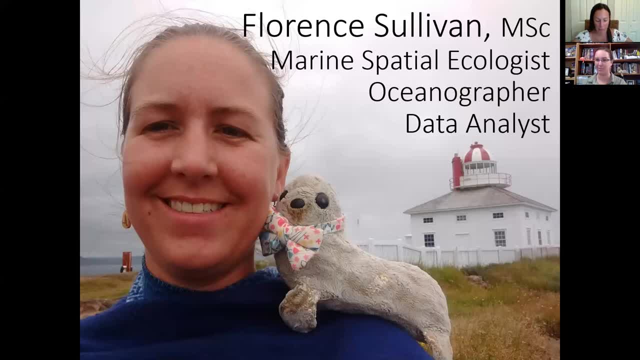 and help us understand the puzzle of our world right now. So I didn't do this alone, And the person, animal, who really got me started on this journey, and that everyone in my family agrees, is my research assistant, Sealy. 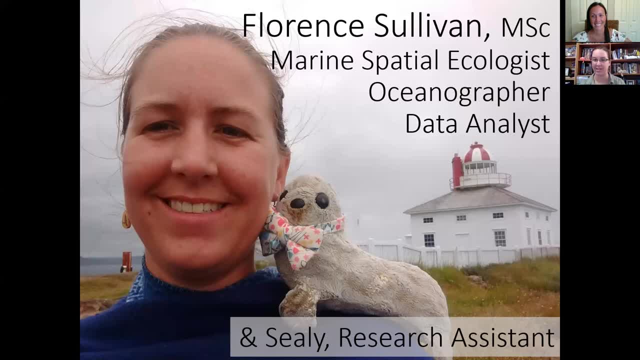 Now, I was very clever, you know, when I was a child and his name is Sealy because he is a seal. So forgive me for my timing, But there we go, And Celie is here with us today. So there you go, He's still around. 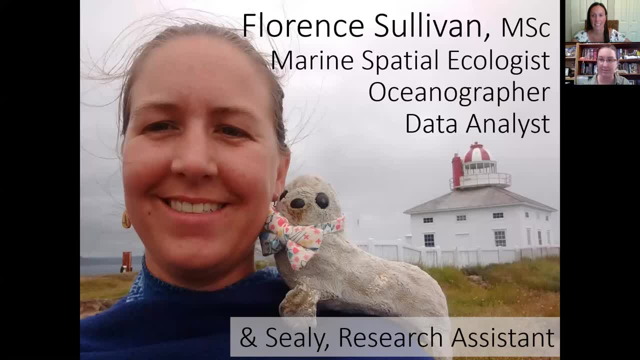 Now I want to give a shout out to my mom, who tracked down a bunch of photos of the early days of Celie and Florence to help me tell this story. So Celie and I started when I was two days old. Celie was a gift from a great aunt And the earliest record in photos that we could find. 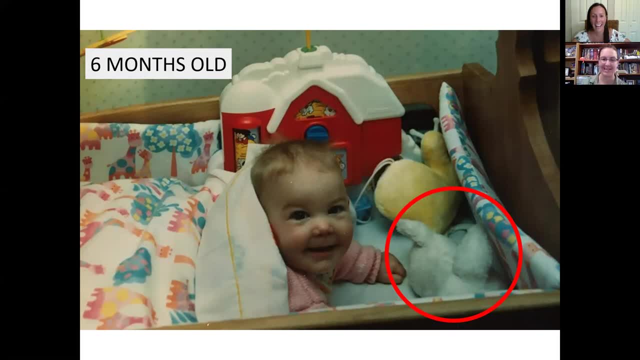 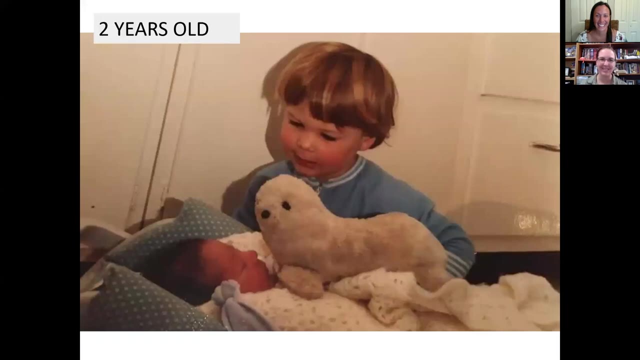 was at six months old. He was a lot fluffier then And a little bit whiter- not quite as gray- And so he was there in my crib And he's starting to get a little shabbier by the time I turned two. 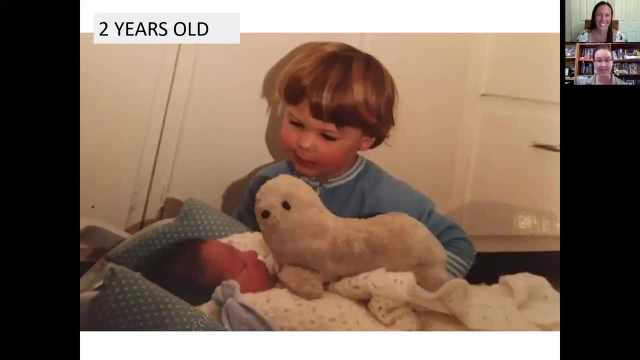 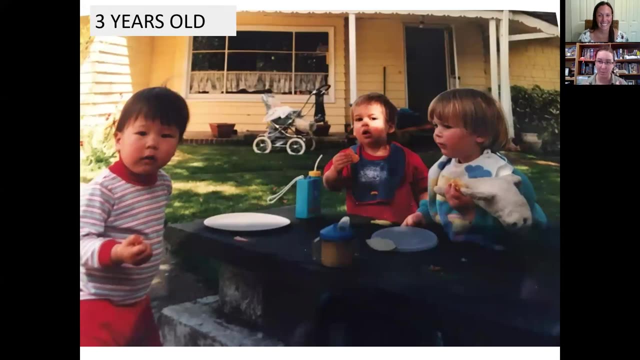 years old and my little brother arrives. And of course my brother had to be introduced to Celie immediately. And just to tell you how important this seal was like, look he's in my arms at a picnic. He doesn't even get to be put down for the important. 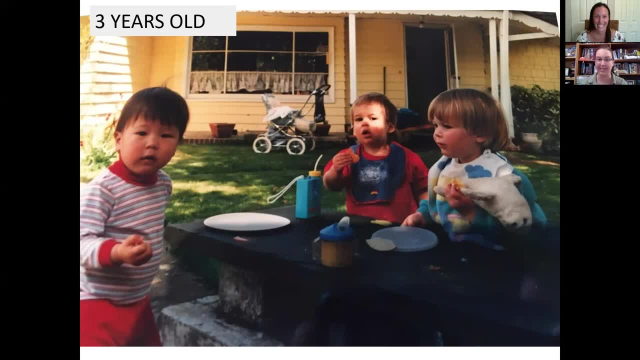 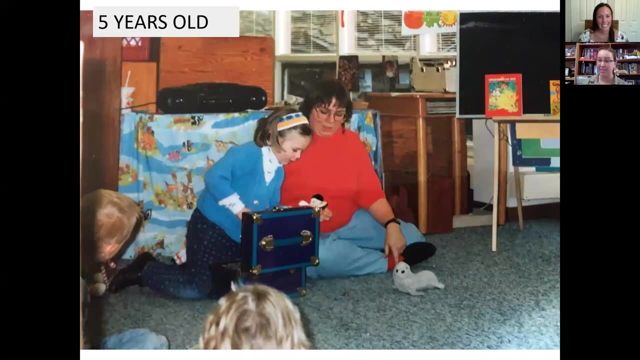 act of eating and of snacking and of, you know, having sustenance. So that's probably why he's no longer as white as he once was was because he's been dragged through everything Fast forward till I'm five years old. I'm in preschool. This is the precious box. This is show. 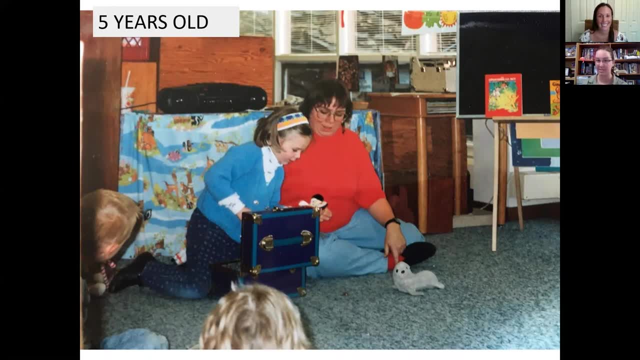 and tell where you were supposed to show the most precious thing to you, to all of your classmates, and to really share something special. So, of course, the first thing in the box is Celie. right, This is who I'm going to share with the group. So at this point, I think it's really astonishing. 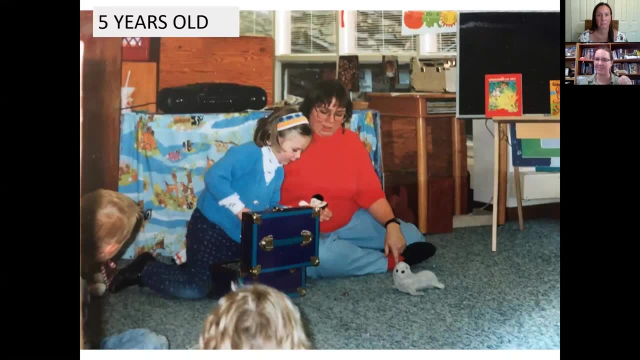 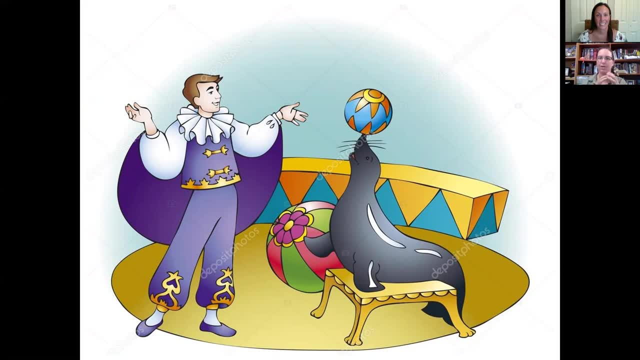 most of my children's books were showing me that seals and sea lions, they're at the circus right. So I was like: all right, if I want to spend time and if I want to have a job with real seals, then I have to go to the circus right. So that was the first career goal that I 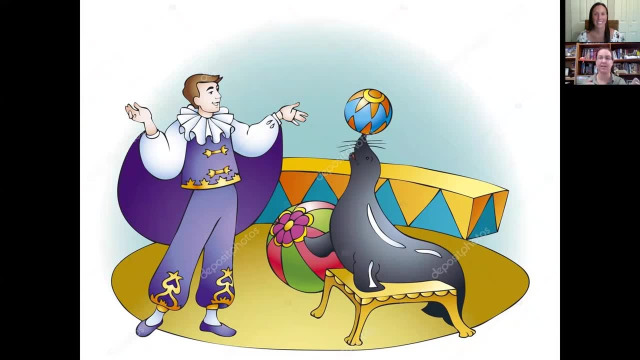 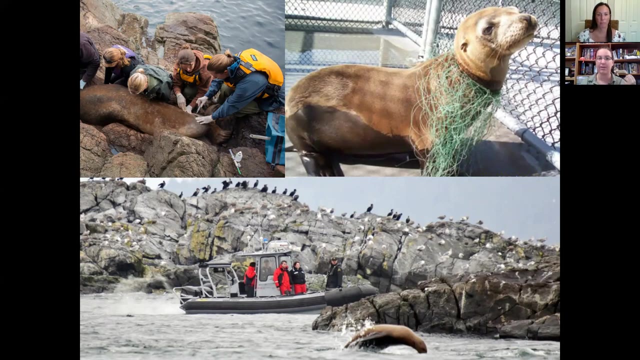 personally remember was I want to spend time with seals, Therefore I have to be in the circus. Very logical, Very logical, right. So turns out that's not the only place that seals exist. When I was in fourth grade, we saw a film in class that had these really cool people in red wetsuits that were going out in 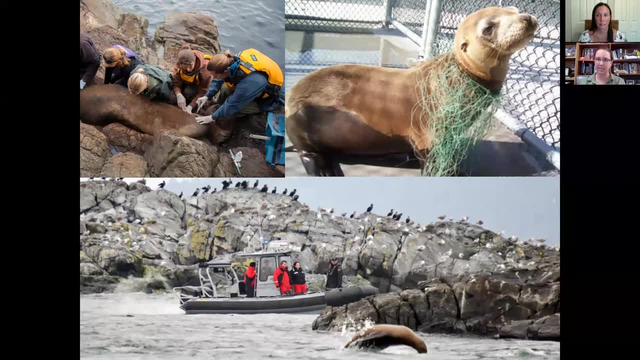 California and finding seals and sea lions that were entangled in fishing nets and cutting them free And and cutting them loose and rescuing them, And I thought, mind blown, that was the coolest possible job And obviously the best way that I could spend the rest of my life, because not only 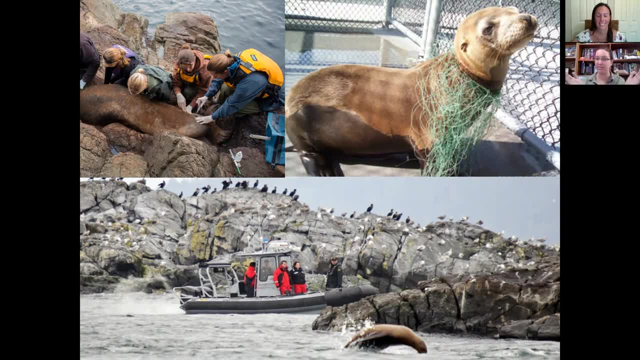 would I be working with seals, I would be making their life better, Right? So that was the first major career switch: From running away to the circus, to working in the circus, to working in marine mammal rescue. And that was fourth grade that you discovered that. 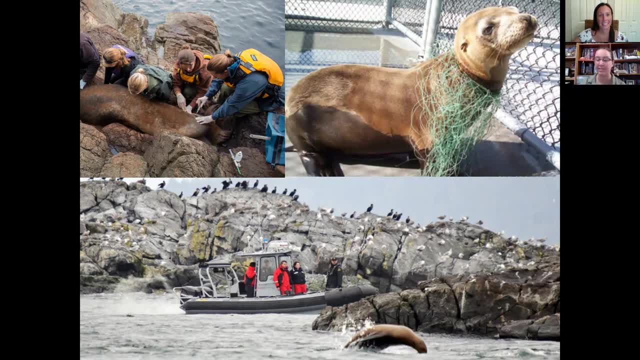 That was fourth grade. Yeah, it was a film in class. you know, they rolled the big TV in the VHS machine on the rolly stand and they shut all the lights off. And you know probably most of my. 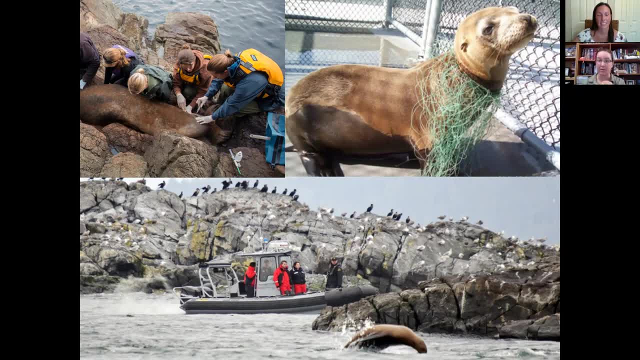 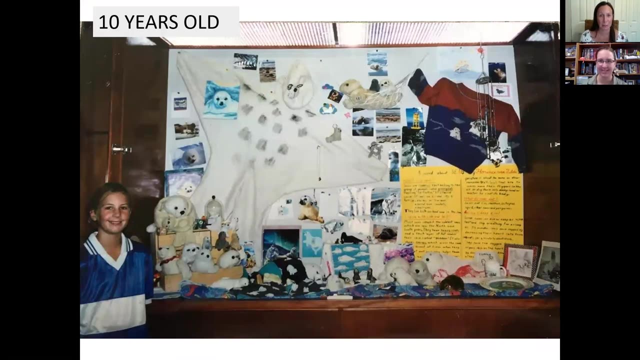 classmates fell asleep because it was warm and sunny, but there were seals on the screen, So I paid attention. Of course, Of course. So there we go. Oh, so quick, I apologize. I always forget to mention something at the beginning, whether it's introducing myself or 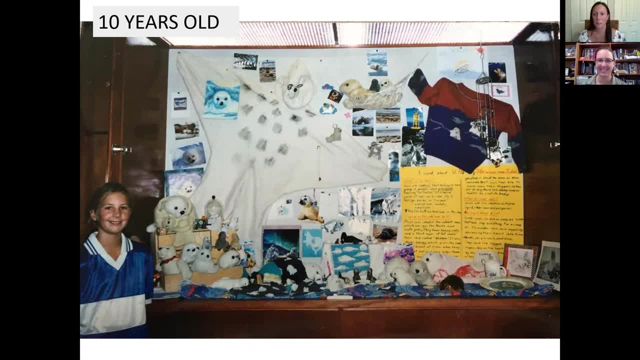 something else. I know I got that one this time, But I forgot to mention for those of you joining us, if you have questions for Florence or Celie, you can ask those whichever way you prefer. We've got the chat in here. we've got the Q&A for those that are with us live right now, And you can also. 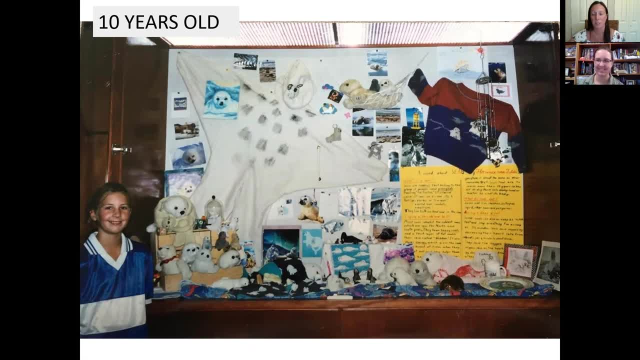 raise your hand if you'd like to speak and actually ask a question to Florence or Celie. So please keep that in mind And we'll make sure we get to your questions as soon as we can. Sorry about that, Florence. That's perfectly fine. It just gives you more time to admire my extensive seal collection. 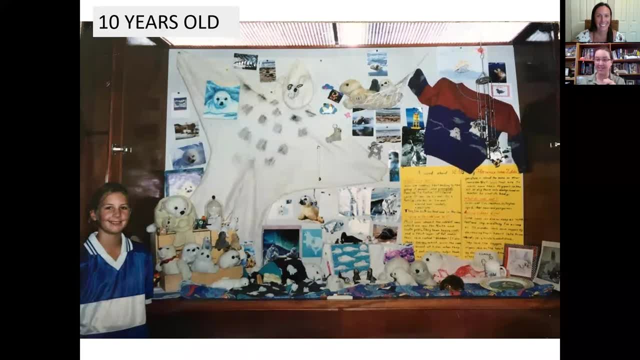 Right. So most of my family had cottoned on to the fact that I was quite obsessed with seals And therefore, as many of you who have ever enjoyed a particular thing, maybe your family decided that you liked small figurines, Maybe you liked dolls. 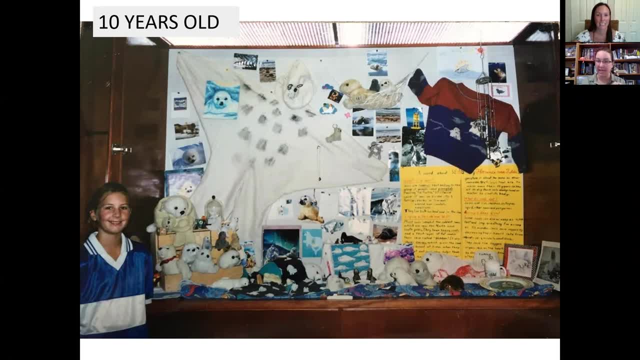 Maybe you liked dolphins. It turns out when you like a thing, your family tends to give you that thing as a present for every possible occasion. And it's the BEST, It's so great. So by the time I was 10 years old, I had written a couple of reports for my science fair and collected a bunch of seal. 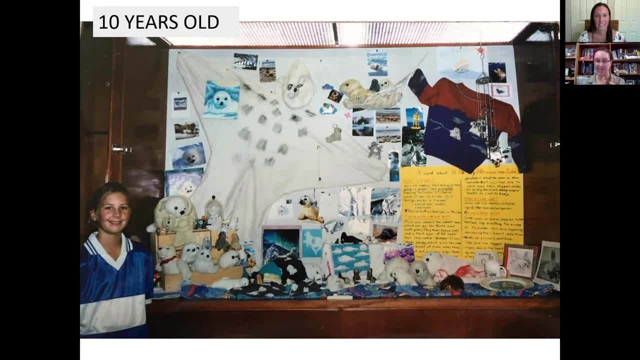 figurines and really started to try and understand how cool were seals and find all the neat facts that I could about them. And my local library had this awesome thing called the seal art book And I where for a month. if you had a collection of something, you could display your collection. 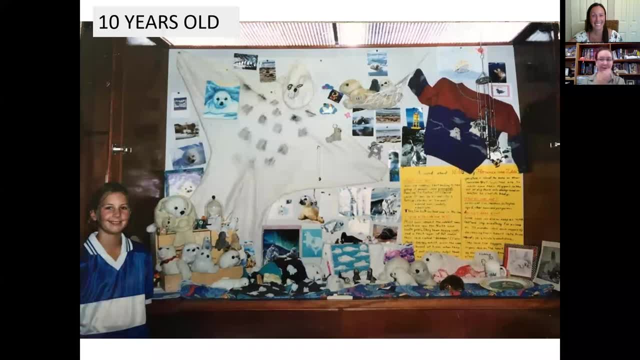 at the library. Yeah, and it would rotate every month and anyone from the community could say I have a thing that I want to share and I'm going to put it up. So this is my collection of seals, with my little fourth or fifth grade science report about seals hanging at my local library. 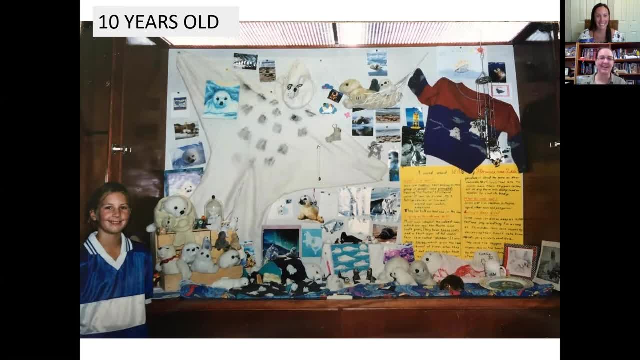 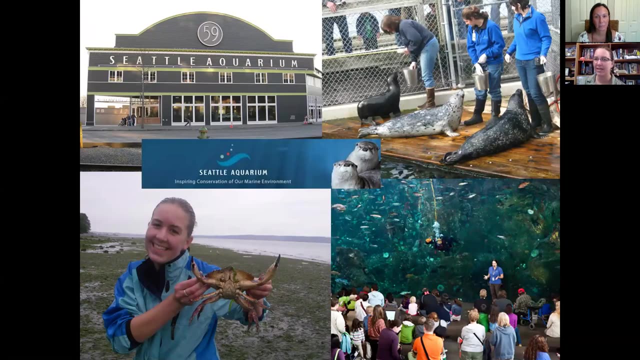 Amazing. Yeah, so at this point, well established, I'm obsessed with seals and I want to work in seal rescue and rehabilitation. Okay, so I figured I have to know what to do, right? And I come from Seattle, and Seattle has a world-class aquarium at Pier 59, and they have a really great 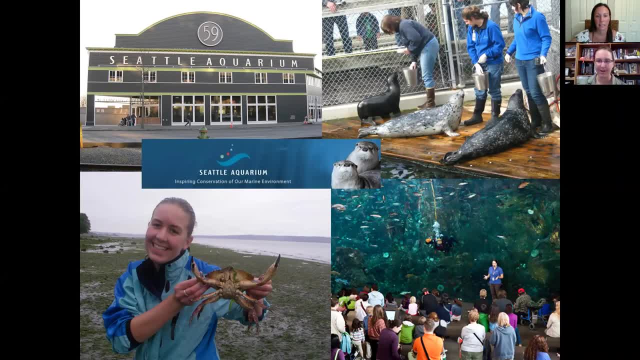 teen volunteer program. So I was so excited about this program and I bugged them so much that normally you're not allowed to go in to participate until you're 16 years old. right Now, my birthday's in May and I managed to argue my way in by saying: hey, I am a sophomore in high. 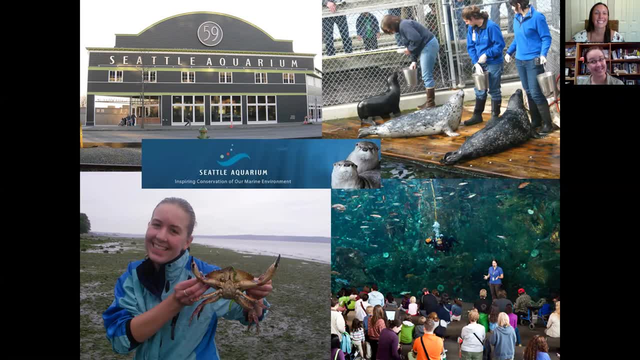 school. I should be allowed to join, even if I'm not 16 yet, because your training is in December and I don't want to have to go in. I don't want to have to go in. I don't want to have to go in. I don't want to have to wait until next year December to be able to start volunteering. I am too excited, So I argued my way in and I spent the next four years. The minimum for the program is coming in twice a month for a four-hour shift. I believe They may have changed that. 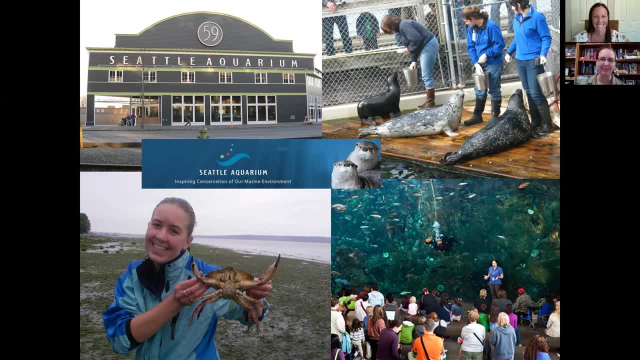 I spent most weekends at the aquarium for as long as I possibly could, And that was a really cool program because it taught me how to be confident in speaking to the public. It taught me how to say I don't know and be okay with not knowing when the public 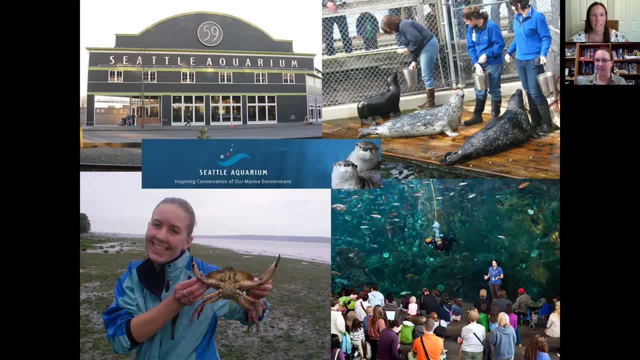 has a question for me, right? This is the basis of research. It's figuring out what you don't know and being willing to go find the answer. That's a really great point. It is a great point, So, recognizing that when someone asks you a question that you don't know. 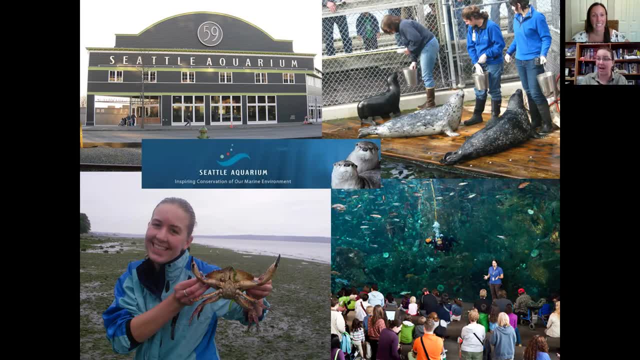 you don't need to make up an answer to sound smarter. You can say: I don't know, Let's go find out together, And that's how great things start right. It takes a lot of people a long time to learn that. Yeah, it's a really great program. They do a lot of mentorship and you 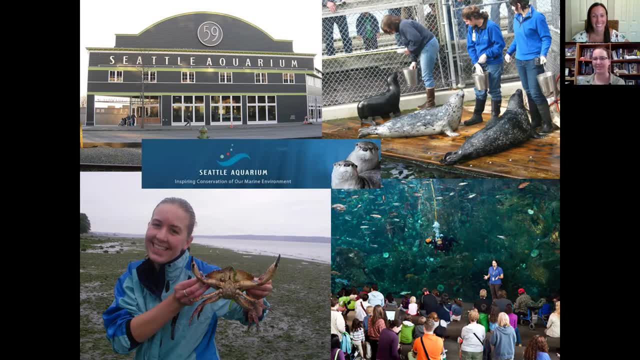 get to hang out with all of the fishes and the marine mammals and really cool people all the time. They have a beach naturalist program in the summertime where you can go down to the low tide and interact with people who are just walking the beach and teach them about the 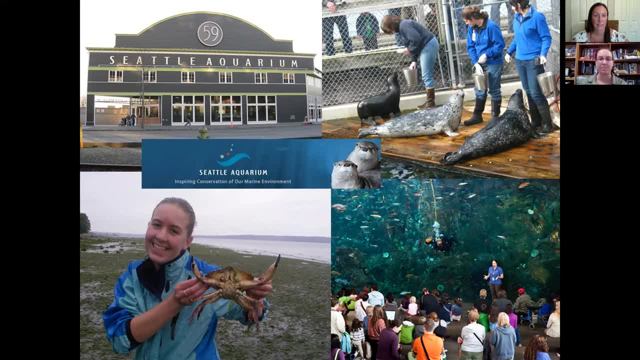 organisms that they're going to find on the beach, And that was a really, you know, formative part of my high school experience. How did you find out about that? Was that just because you had visited the aquarium before? obviously I had visited the aquarium before. yes, But also. 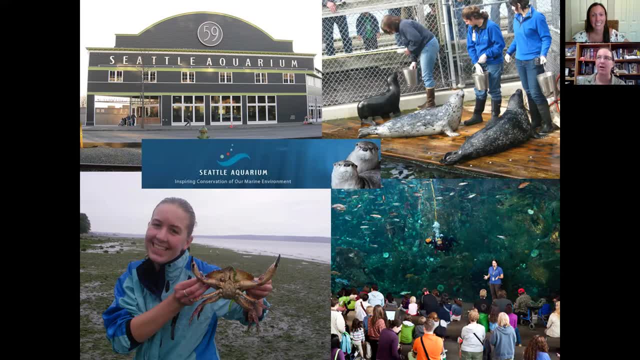 there was a volunteer fair at my high school. We we all had volunteer program sorry projects that we had to complete as part as a service requirement, And so the I think I sort of knew that you could be a volunteer at the aquarium. 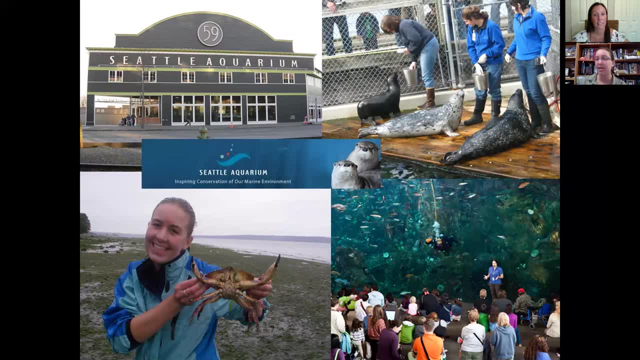 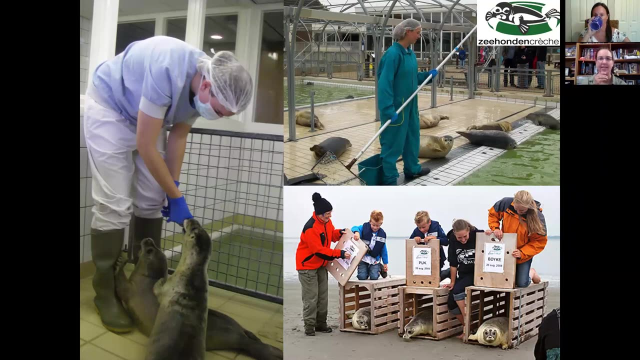 I'm not sure that I knew that as a teen I could do that until they had a table at the volunteer fair at my high school. So, yeah, So that was a big part of high school And and then I graduated and went to college and got to live my dream The summer after. 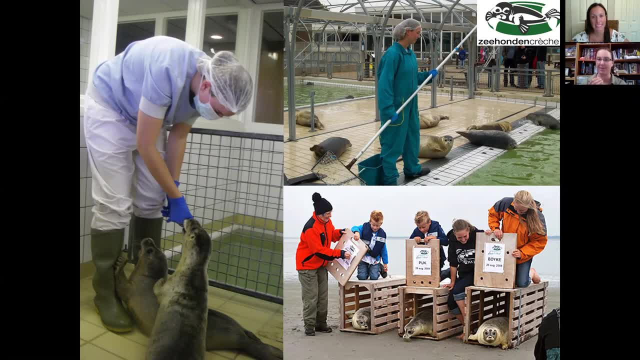 my freshman year at college, my grandmother. we were going to visit her for the summer and she said: I found a thing for you to do while you're visiting me this summer. There's a seal rehabilitation clinic not far. And she emailed them and she called and she 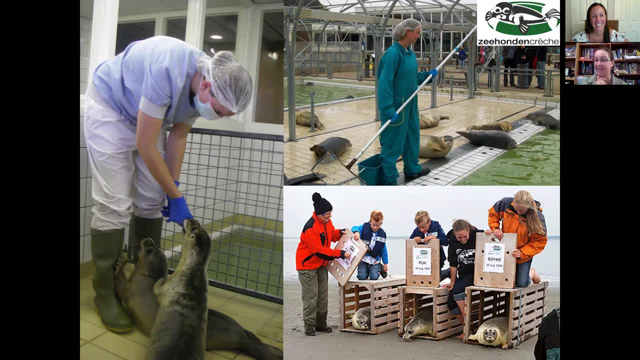 found out about the volunteer program there And I did that and I was like this is a there. and she was like you need my granddaughter to come. you know, as grandmothers are wont to do, and it was the best thing. So here on the screen, on the left side here, this is Sipi and this is 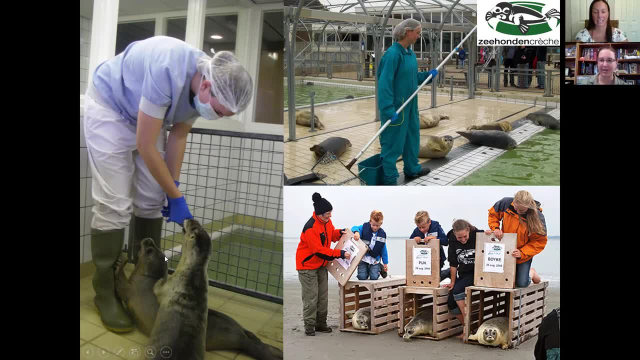 Kai. These are two of the rescued baby harbor seals that I got to help nurse back to health, and this is the first time that I got to hand feed them a fish. They had finally been weaned off of the fish slurry that was helping them put on weight and up in the top corner. 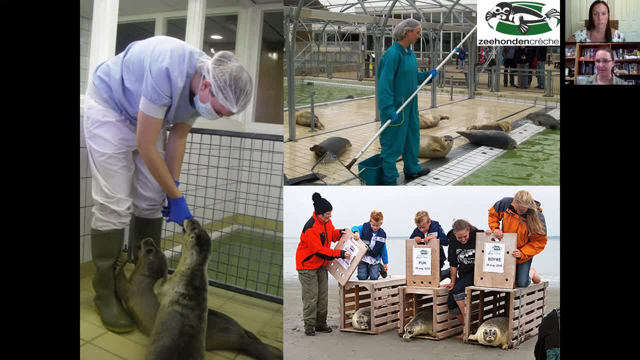 we have some other seals that are well on their way to being rehabilitated and I am scooping fish out of the pool for them, because you can't leave fish in the pool too long, otherwise it will start to have bacteria and that could be not great for the seals. and then down in the right 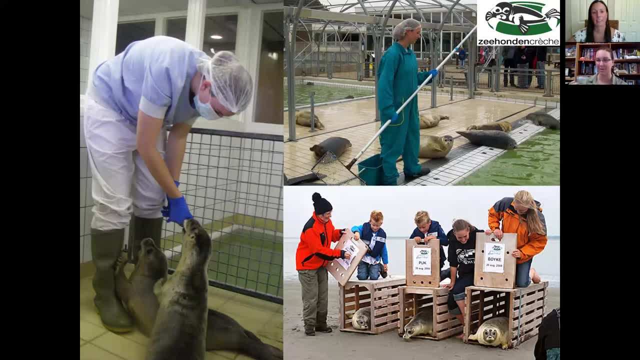 hand side is being able to release the seal pups once they're all healthy. So I spent two and a half months at the Zeehondekrish in the Netherlands helping to rehabilitate seals, and it was a dream come true. I met some fabulous people. 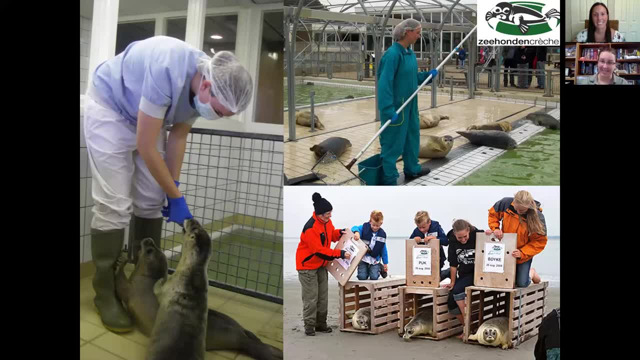 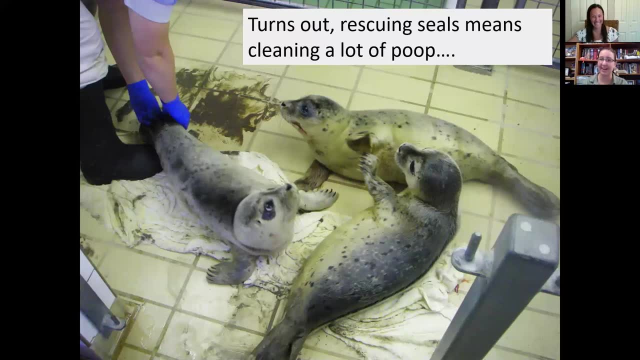 I learned a lot of things, but I also learned that it turns out rescuing seals means cleaning a lot of poop, and three quarters of the job was sanitizing and cleaning the rooms and, yeah, doing lots and lots of laundry- The stuff no one tells you about. 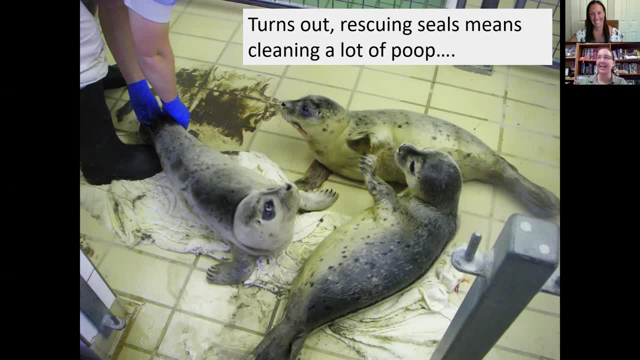 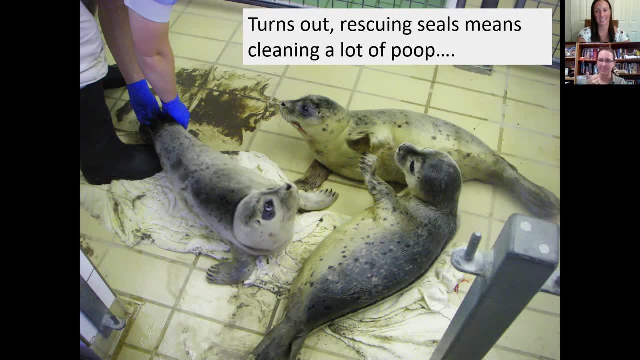 I loved seals but I wasn't fond of the idea of doing laundry and cleaning poop for the rest of my life. That the program I was in was not a veterinary program, which would be the other way of getting in and doing more with the seals. that had more to do with caring and less to do with. 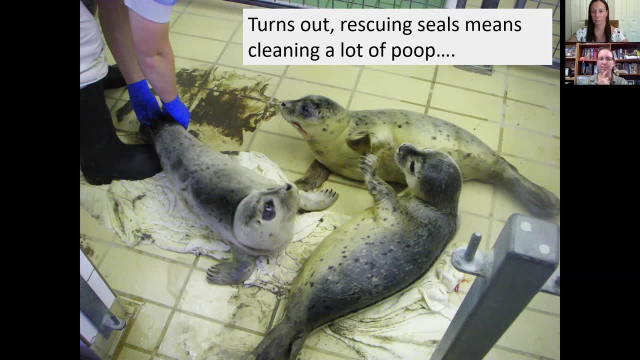 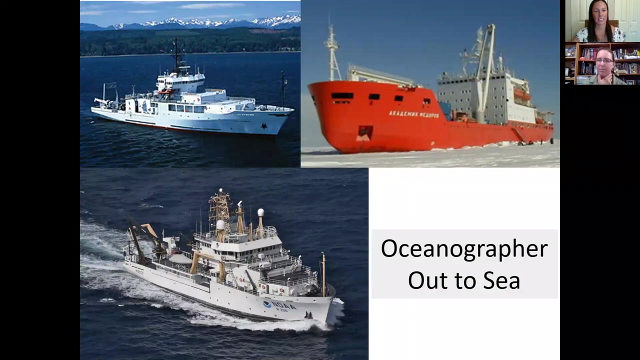 cleaning up all the poop. So I was a little bit lost, you know. So I had to completely rethink what I wanted to do once I realized that this was not my career path anymore And I had to reinvent myself. So what did I do? I threw myself into my undergraduate program at the University of Washington in Seattle. 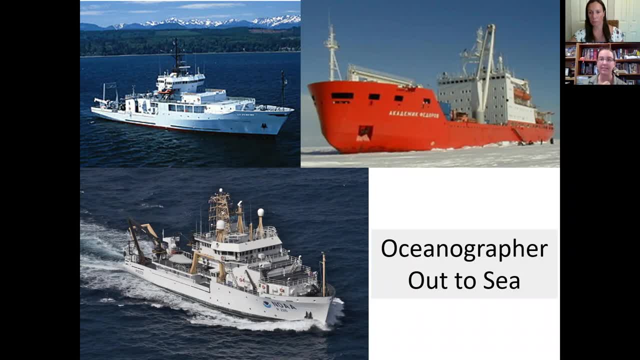 I was in the oceanography program And I went out to sea right Now. oceanography is the study of the ocean And to get started here you have to know the biology, the geology, the physics, the chemistry and you have to take 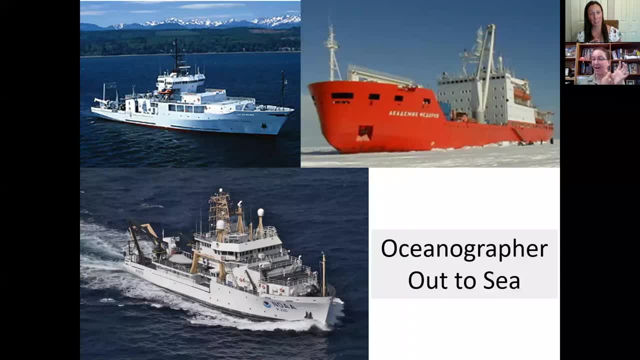 calculus and do a bunch of math. The other things that they don't always tell you right? The other things that they don't always tell you before they even let you take the classes, about how all of those things work in the ocean, right? 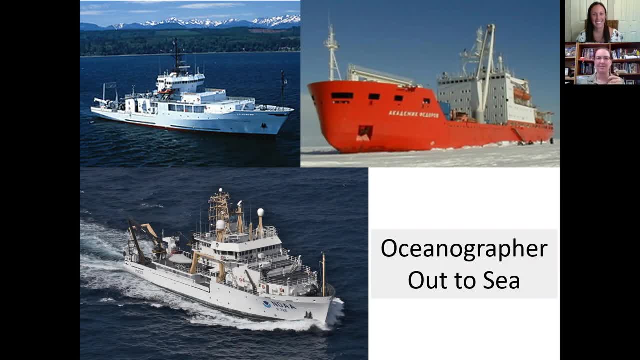 So it's a very science-heavy degree, And in high school I had taken as many science classes as I could because I knew that that was going to be important. But this rammed it home even further, right. So I dove into the science and as soon as I got out on the boats I was like